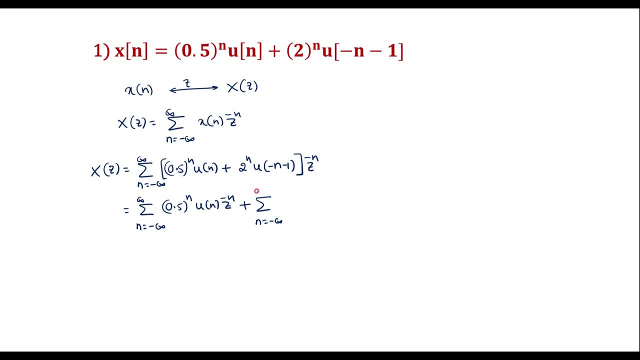 similarly, n is equal to minus infinity to infinity: 2 power n? u of minus n minus 1 z power minus n. let me simplify this further, or i can represent this as summation here: u of n indicates the signal is right sided signal. for n less than 0, the value of the signal is 0. 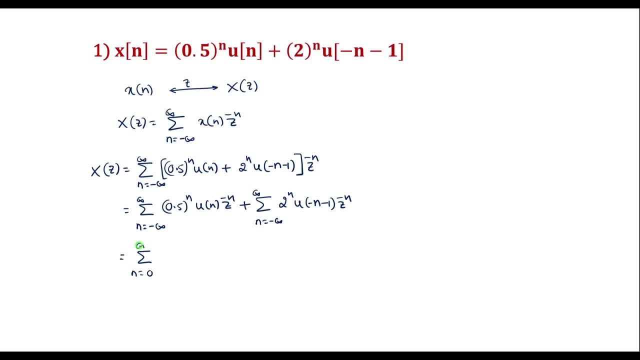 therefore n varies from 0 to infinity. 0.5 z. inverse power n. similarly, here u of minus n, minus 1 indicates that the signal is left sided signal, and it varies from minus infinity to minus 1. that is, for n greater than minus 1 the value is 0. therefore, here n varies from minus infinity to minus 1. 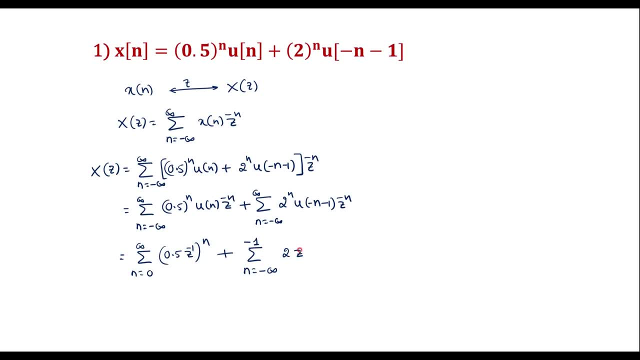 we have 2 z inverse power n. further i can simplify this as summation: n equal to 0 to infinity, 0.5 z inverse power n. plus. here i can represent this as n is equal to infinity to 1, if i consider n as: 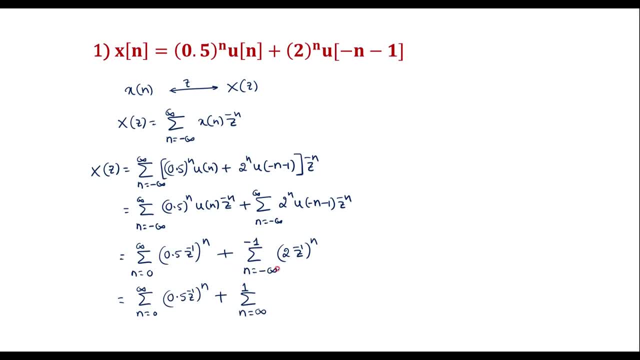 a positive values of limit, then we supposed to replace this n by minus n, that is, 2 z inverse power minus n, which is same as this expression. let me continue here or i can write it as: x of z is equal to summation, n is equal to 0, to infinity. 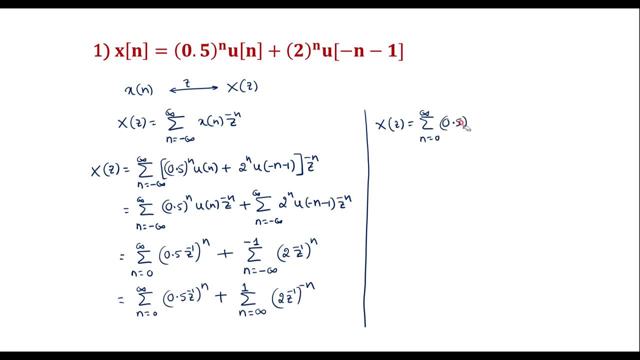 f, x0 to 0.5, x0 to infinity, sort of a loss. thechez arrival, manifestation of the infantry. answer: if we have zo, that is Terrorism. you have to believe that thehour meeting that is agriculture, or true or false, or true? mäster Cućilo, when u replace this And ersch thirty of the moment, that returns minus n as positive point, which is zero. if you compute this gets alpha minus minus that it thethoseこ. 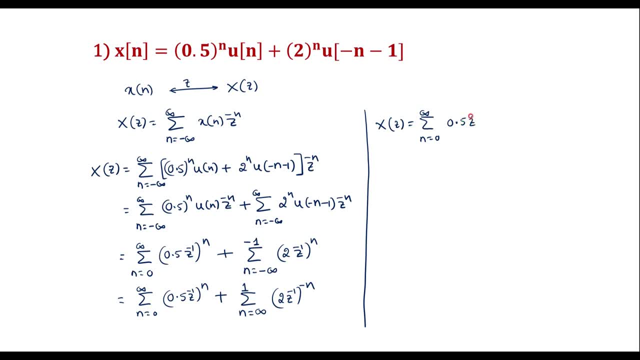 0.5 z inverse power n plus summation n is equal to 1 to infinity. Here this can be represented as 2 inverse z power n. We know that summation n is equal to 0 to infinity. alpha power n is equal to 1 upon 1 minus alpha and summation n is equal to 1 to infinity. alpha power n will. 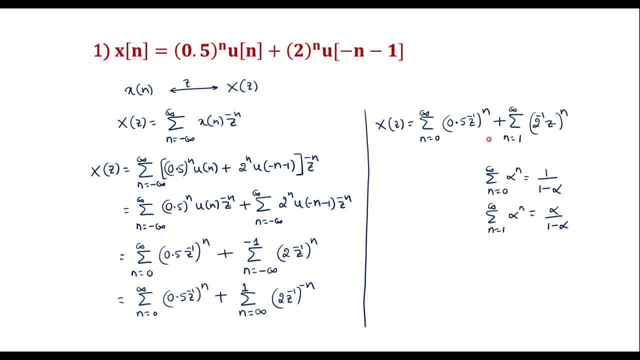 be alpha divided by 1 minus alpha. Now let me apply these two formula here. Therefore I can write: x of z is equal to here. alpha value is 0.5 z inverse, that is 1 upon 1 minus 0.5 z inverse. 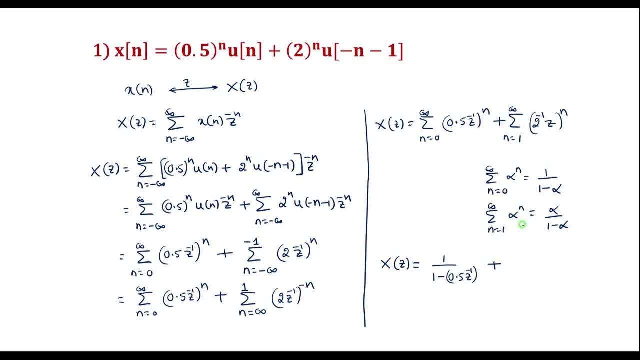 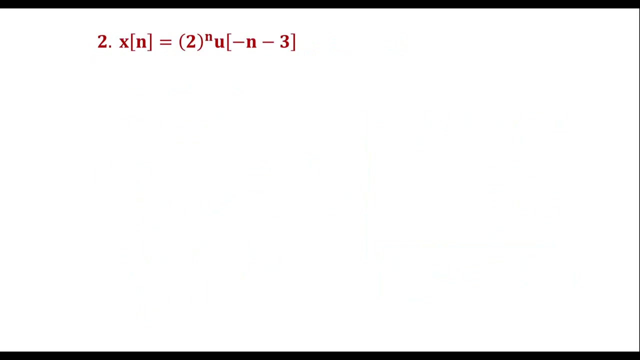 power n. plus here we have alpha. Alpha is 2 inverse z. 2 inverse means 1 by 2 z divided by 1 minus 1 by 2 z. So this is the z transform of given function. Let me consider the second example. So x of z is equal to summation, n is equal to minus. 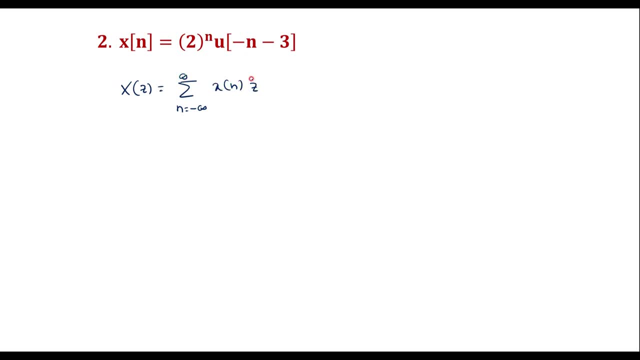 infinity to infinity. x of n, z. power minus n, or we can represent it as: n is equal to minus infinity to infinity. Here x of n is 2. power n? u of minus n minus 3. z. power n? Here? u of minus n minus 3 indicates that the signal is left sided signal and which. 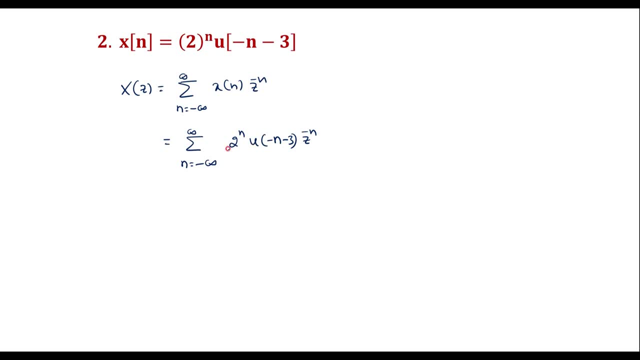 starts from n is equal to minus 3 up to minus infinity. It means the n varies from minus infinity to minus 3.. Therefore, I can represent it as: summation n is equal to minus infinity, to minus 3. 2 power n, z. power minus n. or I can represent it as: summation n is equal to: 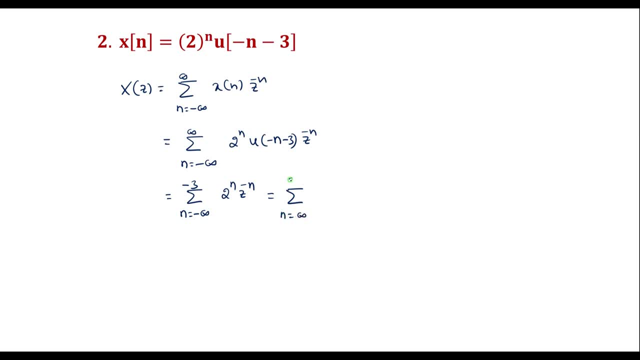 plus infinity to 3, provided that I will replace n by minus n, which is same as this one, that is, 2 power minus n, and this is z power n, or I can represent it as: summation: n is equal to 3 to infinity. Here we have 2 inverse z power n, So simplifying. 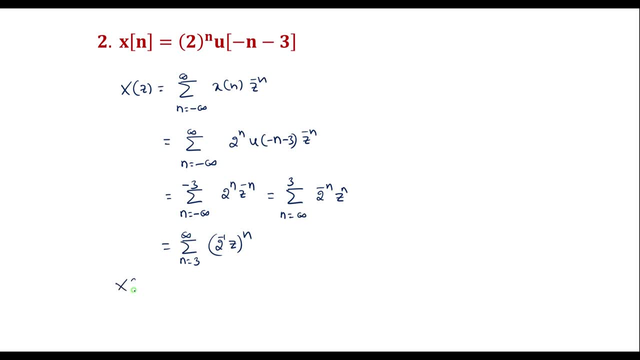 this I will get: x of z is equal to. so here n is equal to 3, that is alpha power 3 divided by that is summation. n is equal to 3 to infinity. alpha power n is equal to alpha power 3 divided by 1 minus alpha. Similarly, here alpha value is 2 inverse z. 2 inverse means 1 by 2 z power. 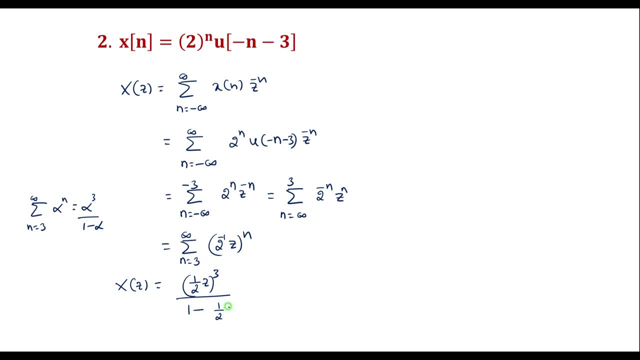 3. minus 1 by 2 z. So this is the z transform of given signal. Now let me consider the third example. x of n is equal to sine pi, n by 8 minus pi by 4 u of n minus 2.. So here I can. 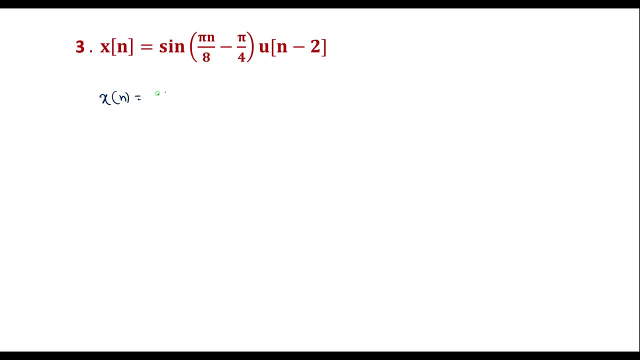 represent this x of n. as x of n is equal to. we have sine here. I will represent it as pi by 8 n minus 2, which is same as pi by 4 u of n minus 2.. For easy simplification, we will solve this problem using z transform properties. 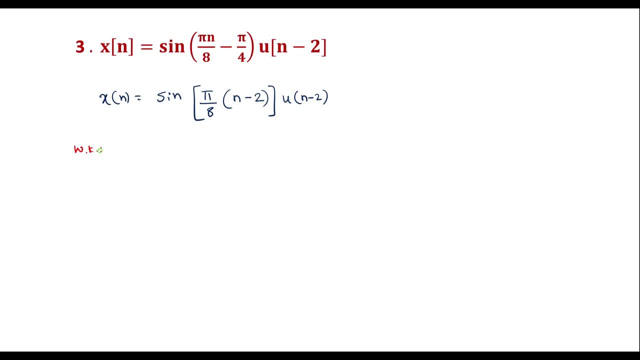 We know that sine omega 0 n? u of n, its z transform is given by sine omega 0 into z inverse, divided by 1 by 2 z. So this is the z transform of given signal. Now let me consider the third example. x of n is equal to sine pi n by 8 minus pi by 4? u of n minus 2.. So here I can. 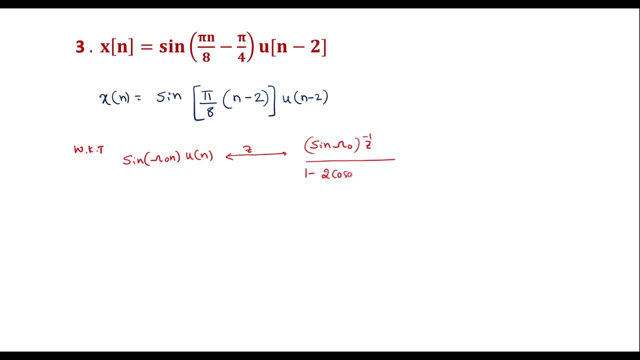 write sine pi n by 8: n minus 2, cos, omega 0, z inverse plus z, power minus 2 having ROC greater than 1.. So here 1 should remember this formula. Now I can write sine pi by 8: the Z transform of this will be: that is U of n, U of n, the Z transform of this will: 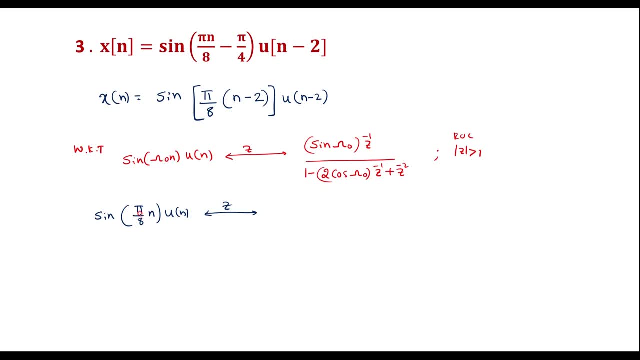 be here. omega 0 is nothing but pi by 8, I will replace omega 0 by pi by 8, so that I will get sin pi by 8 Z inverse divided by. we have 1 minus 2 cos pi by 8 Z inverse plus. 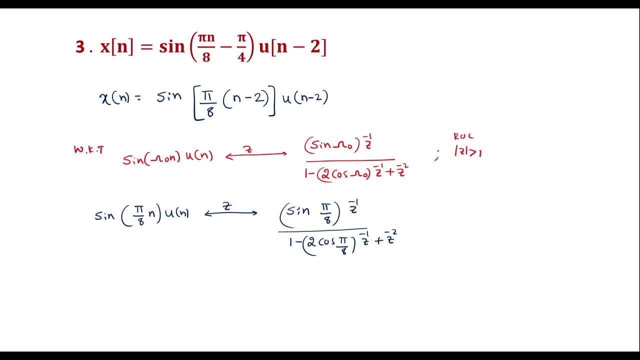 Z power minus 2.. Now by using time-shifting property, that is, use time-shifting property of z transform, I can write it as sine pi by 8. n is replaced by n minus 2, n minus 2, u of n minus 2. 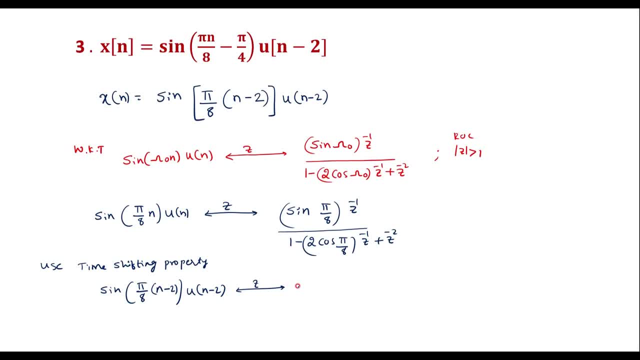 the z transform of this will be: that is shifting property shifted by 2 units. so we supposed to multiply this entire term by z power minus 2. as it is shifted by 2 unit, z power minus 2, the remaining term will be as it is. that is, sine pi by 8, z inverse divided by 1 minus 2, cos pi by 8. 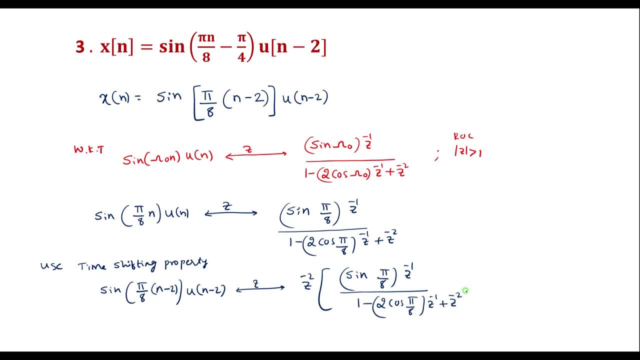 z inverse plus z power minus 2. this is the z transform of gilbert's equation x of n. thank you for watching.